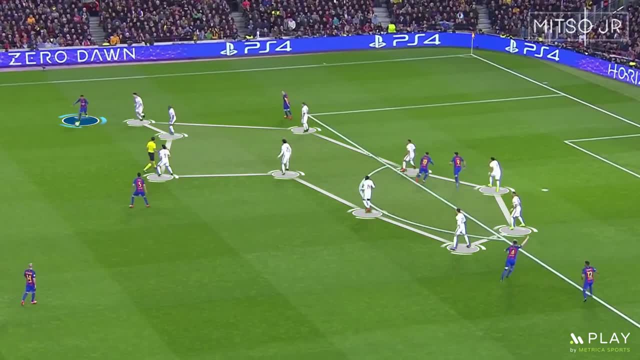 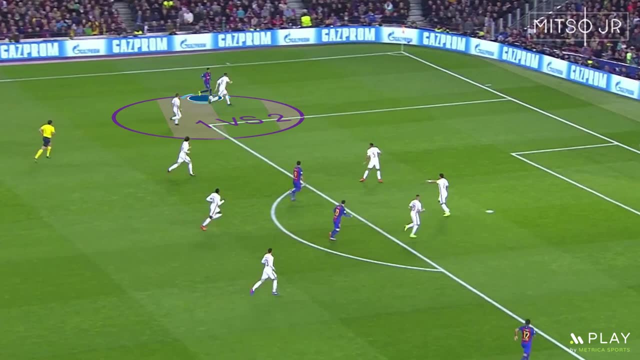 he would always try to go for any possible through-passing options to help progress the attacks as quickly as possible. As PSG were up, they were trying to force Barcelona to keep possession and build their attacks slowly. Neymar was trying to go for the opposite of that by. 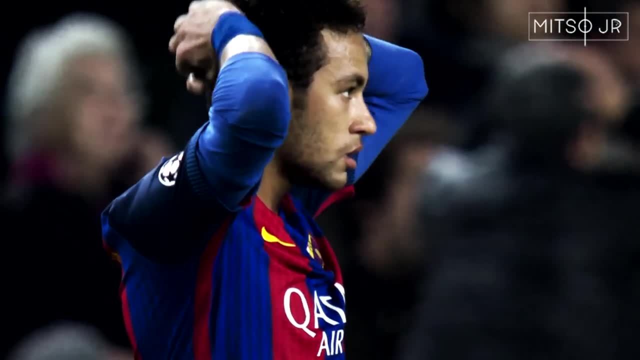 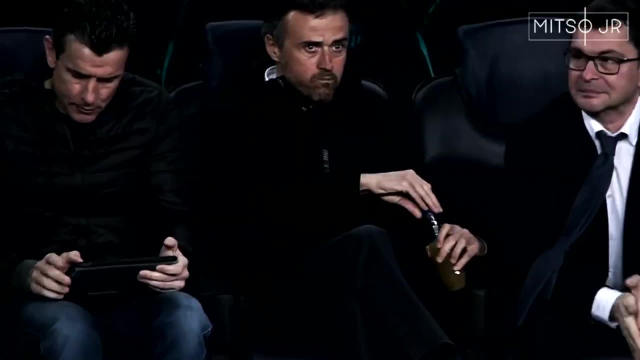 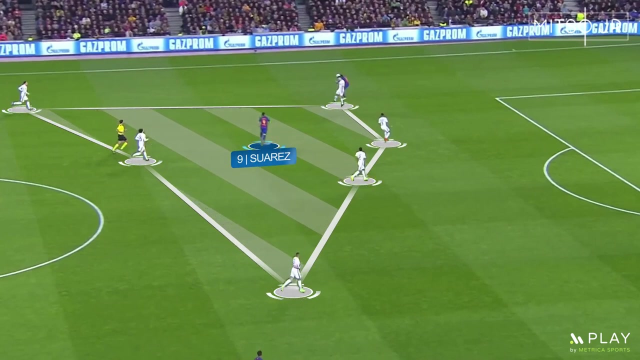 covering passes between the lines, And again, this doesn't work every time, so he played a lot of missed passes in the process. As a wide midfielder, he also had the usual responsibilities of connecting with the striker whenever the defenders go for a long pass. 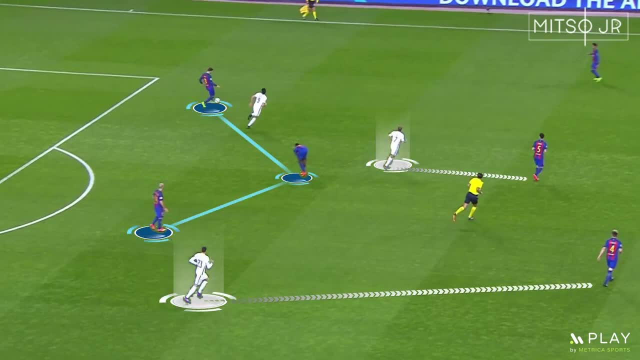 or drop down to receive the ball from them. if PSG applies pressure In those scenarios, he didn't go for the through balls, but instead, as Paris Saint-Germain are pressing with numbers, he would go for a long pass. He would also try to get the ball to the. 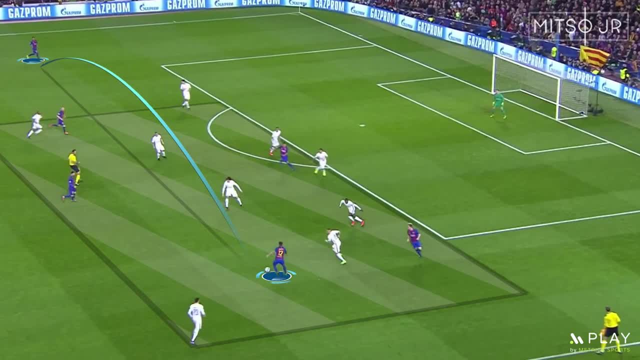 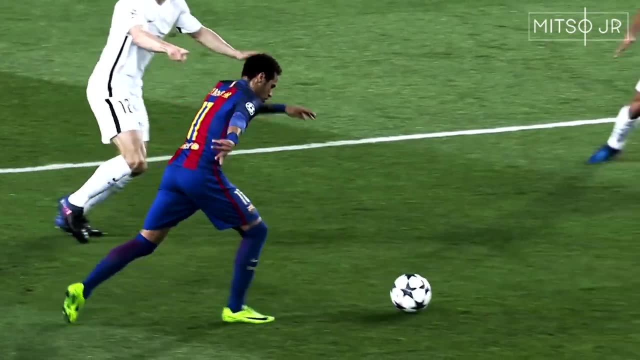 right side and carry it forward. Rafinha was playing with the right-hand side in that game. He linked up with Neymar in multiple occasions to counter Paris Saint-Germain's low-zonal defensive system by switching the play. Neymar was always looking to create the 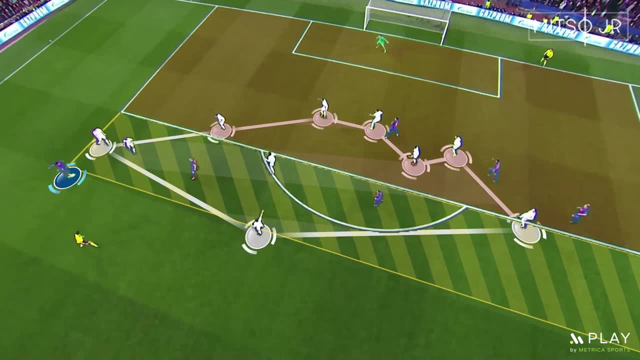 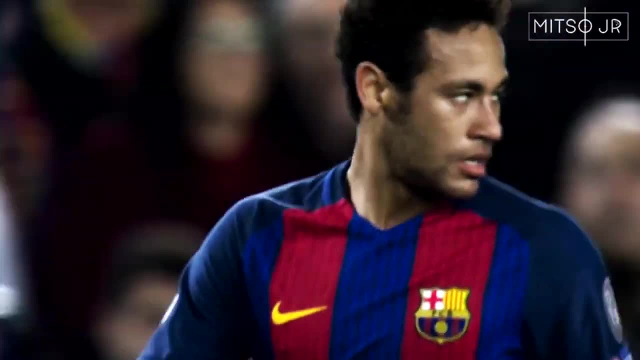 difference whenever he had the ball in his feet. So by reading the situation here, for example, seeing that all 10 players from Paris Saint-Germain are behind the ball- he decided to go for the long shot, which is a very good decision to make in this case. This video is brought to you by Play. 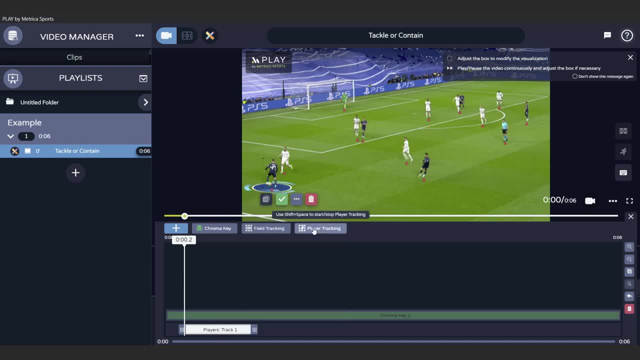 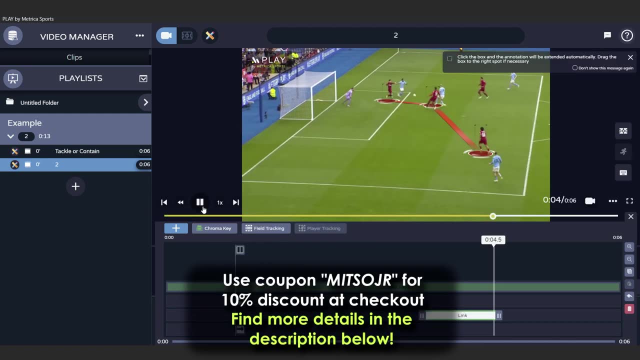 Biometrica Sports, the fundamental tool for every coach and analyst. Create and manage all your video analysis in one platform. Use the coupon Mitsujr at the checkout for a 10% discount. Barcelona were applying high pressure whenever the opposition was trying to build up from the back. 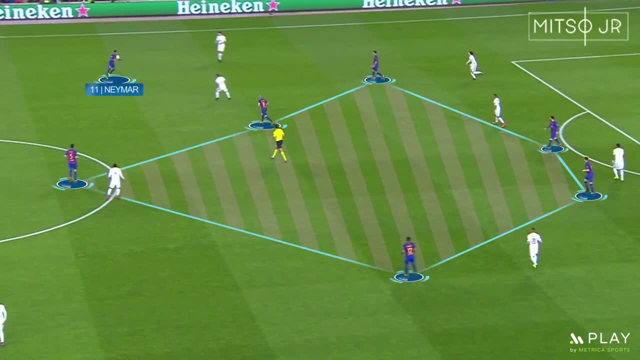 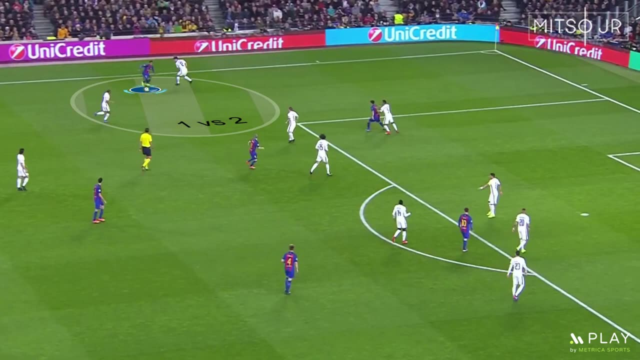 Neymar had the responsibility of trying to intercept the long balls that PSG were forced to play. With the ball, he was always trying to drive forward and connect with his teammates with one-two passes to lose his markers. Realistically, and since PSG had all their 10 players defending, 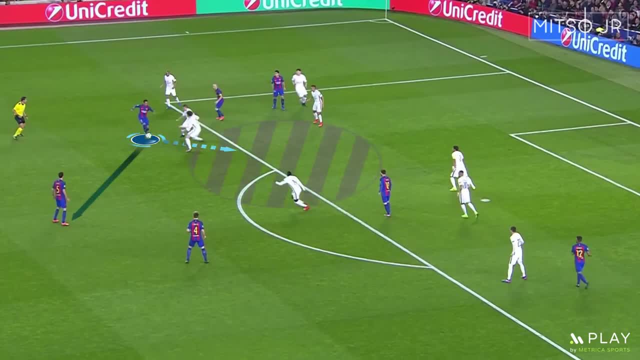 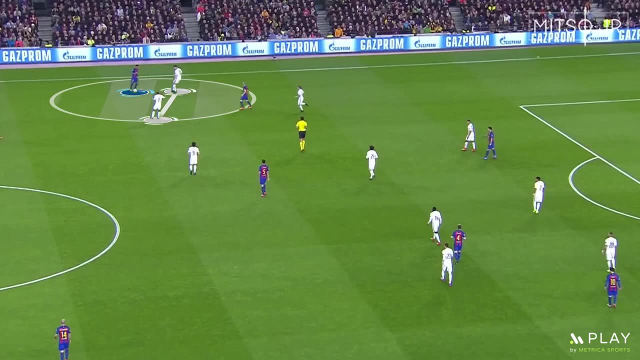 everyone from Barcelona was marked, So he had to take the edge from his off-the-ball movement in between the passes. By having so much time on the ball, even when marked by two or more players, Neymar started to annoy the opposition, which resulted in his markers getting more physical. 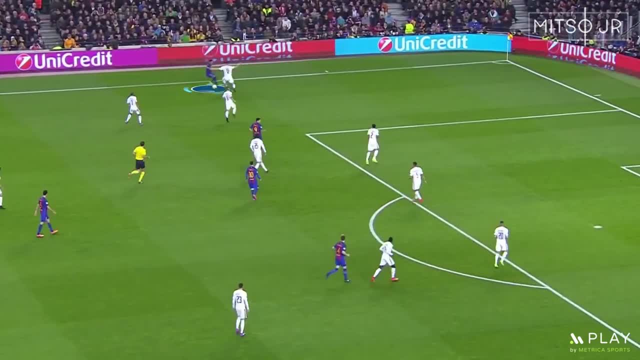 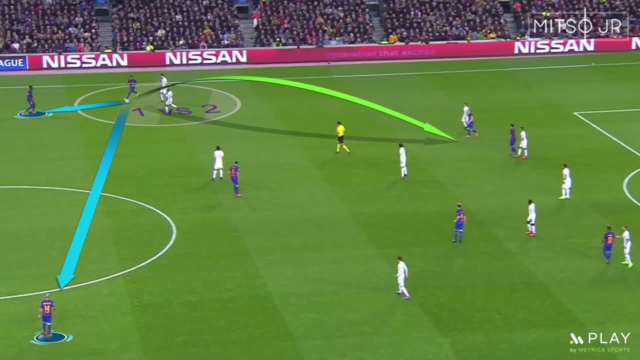 in an attempt to disturb him whenever he has the ball and try to push him backwards. This allowed him to win multiple fouls, but he was always going for the forward passes And that's exactly how the goal was scored. You can see here how he has two back and safe passing opportunities with the. 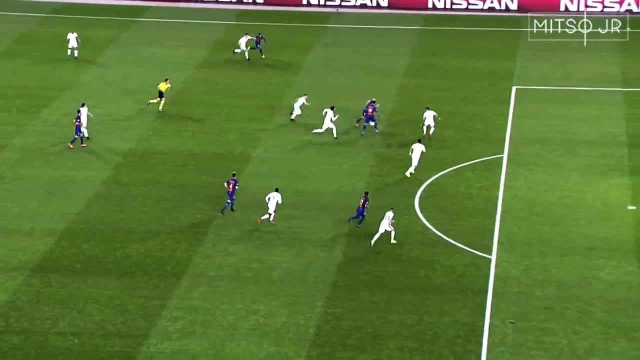 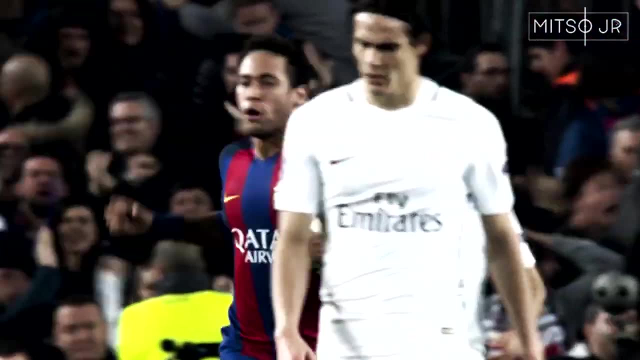 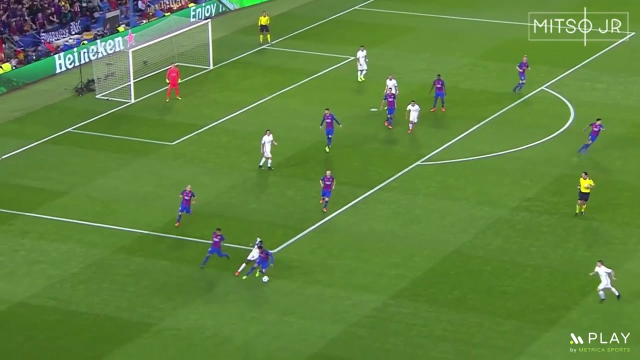 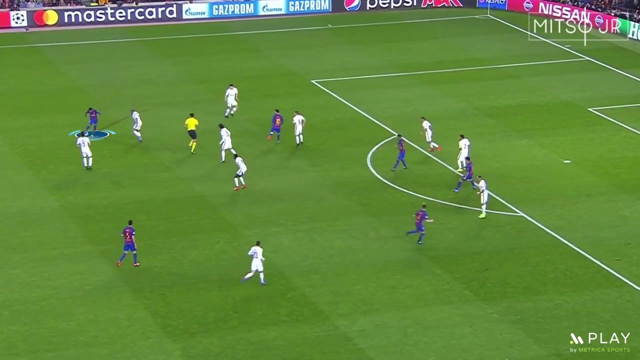 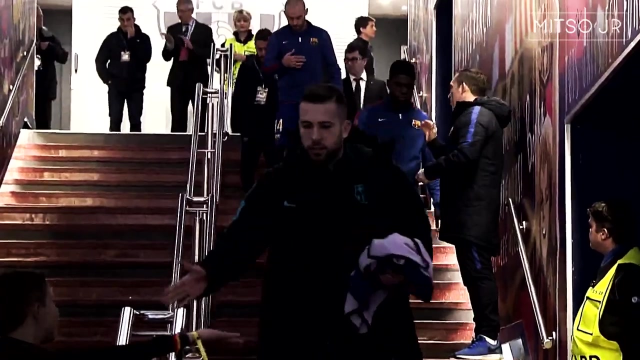 opposition, trying to push him even more. Yet he went for the forward passing option and Barcelona scored. So two main concepts to take in from the first half: His high wall create and his continuous attempts to play only forward passes and avoid negative possession In such big games. the half-time talk from Luis Enrique surely had an impact on the team's 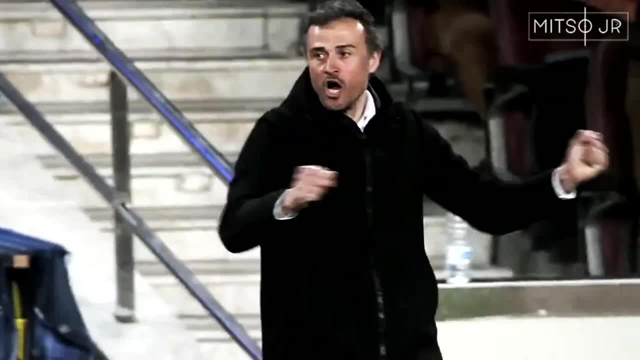 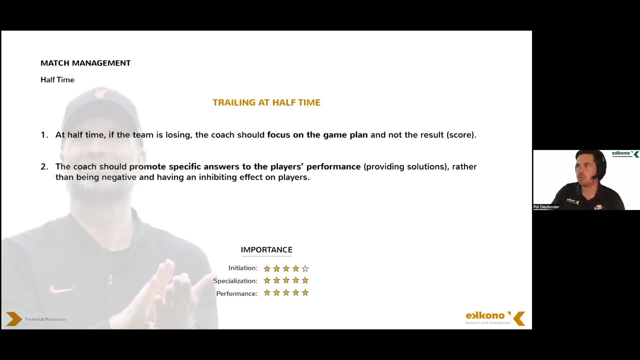 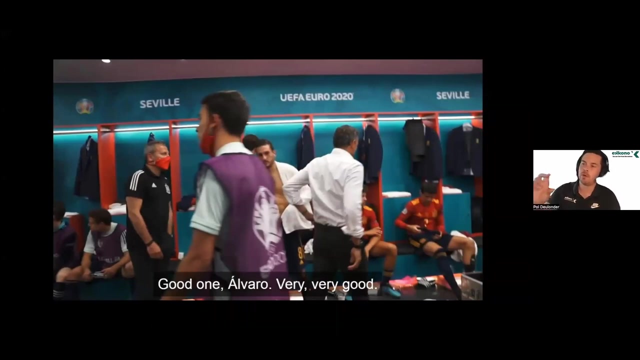 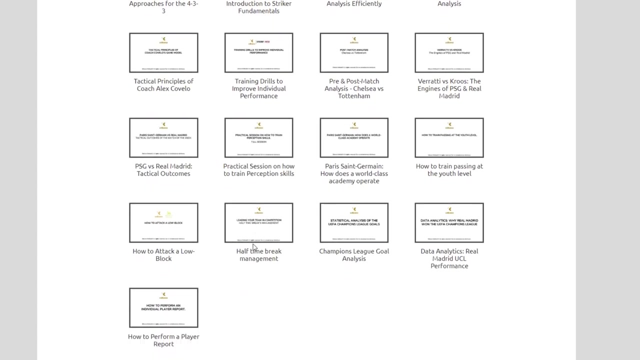 incredible performance in the second half. Let's hear from the Econo Coaches Academy about it. I strongly recommend that you guys watch this full webinar, as they showed detailed theoretical plans to what to do when you are winning or losing, And even showed a couple of examples. 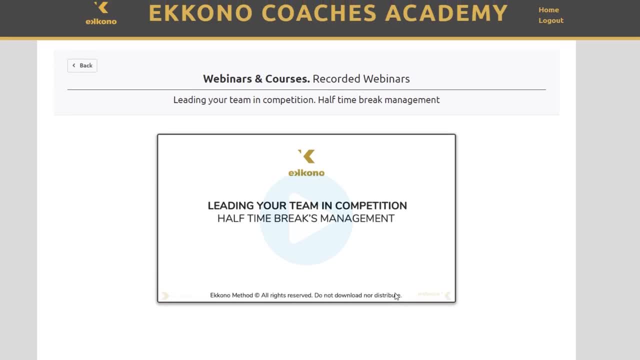 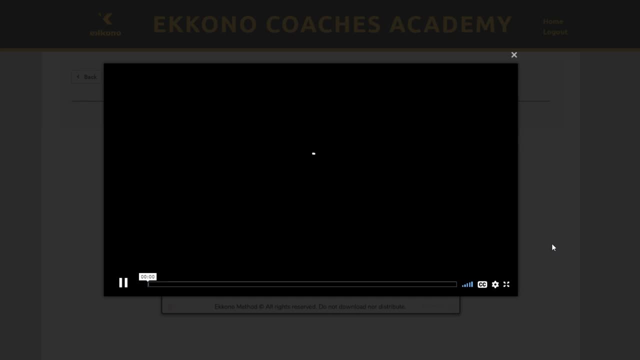 You can sign up totally for free using the code MITSUJR from the link in the description to start watching directly. You will also gain extra benefits and discounts moving forward. Heading into the second half, and the main change here was the fact that Unai Emery wanted to avoid. 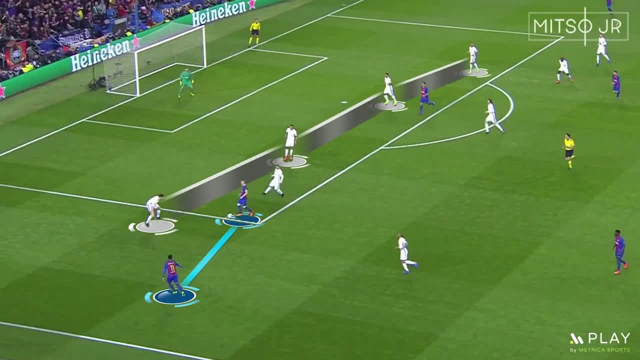 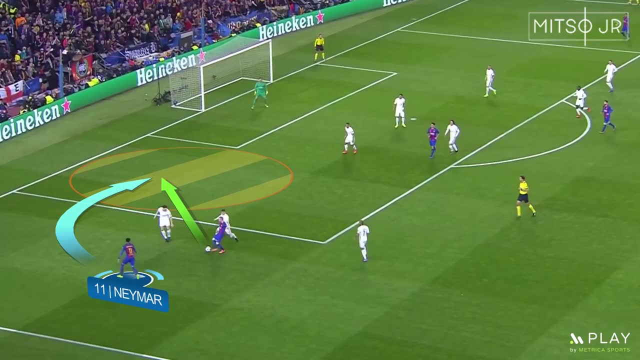 messing things up, So he decided to play with four only at the back. This was a game changer for Neymar, as he now enjoyed huge spaces that he never had during the first half And, right off the bat, he won a penalty after linking up with Iniesta on the wing, Enjoying his first 1 vs 1 situation. 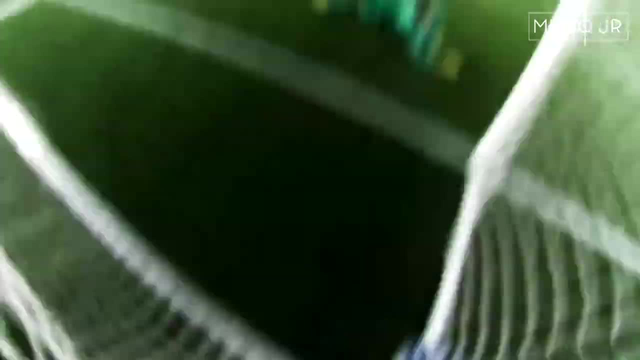 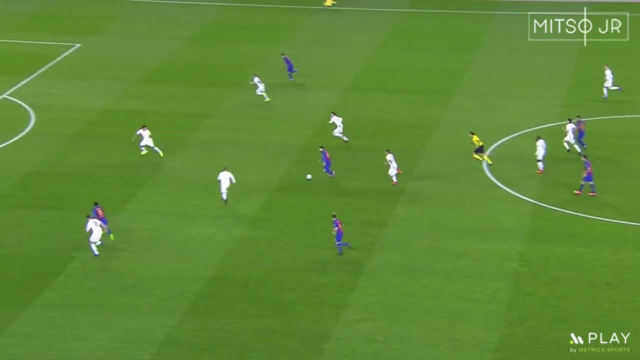 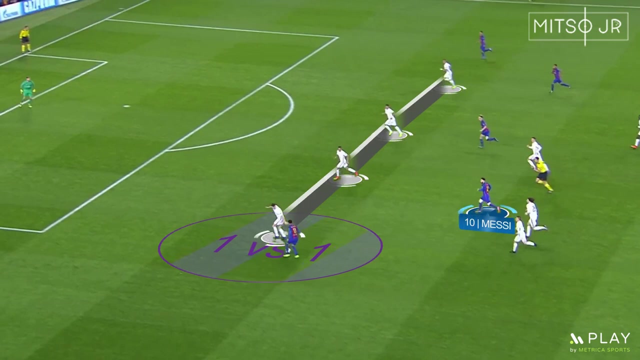 The 4 at the back from PSG allowed Neymar to start linking up directly with Messi. as Barcelona started to have more time on the ball in the midfield, We never saw Neymar being mocked by one player only throughout the first half, But Cavani scored to make it 3-1 and, accordingly, PSG started moving. 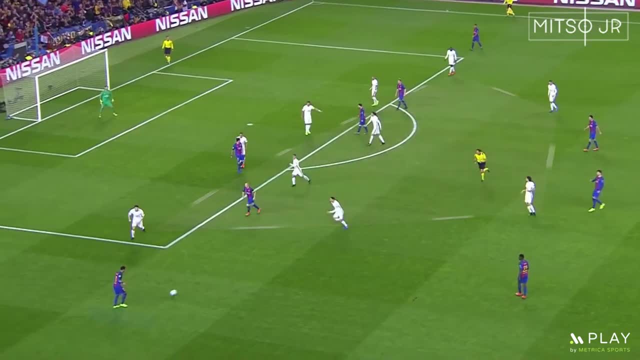 backwards again. However, this time Unai Emery didn't want to replicate what happened in the first half, so the team was trying to perform solidly, Not to have the same situation again. The top 3 had a very good performance in the last half, but then the two teams fell back. The 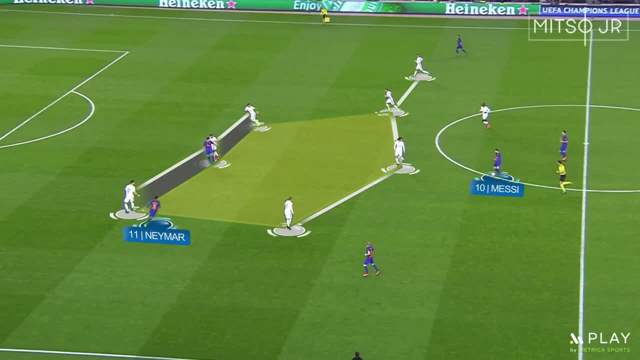 best thing about this was the opportunity for Neymar to be on the rink for the league. One was to get better, but the other was to be a little earlier than what had been expected, so he had to be quite confident, was trying to perform some attacks as well, making the defensive face unstable. 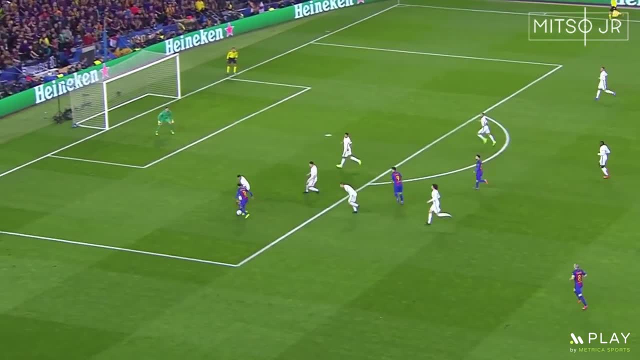 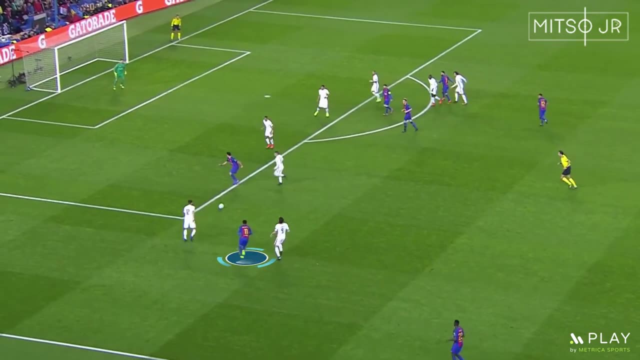 With Neymar having the freedom of moving anywhere he wants. on the left flank, he started creating many linkups with Suarez as well. We also started seeing him cutting inside a little bit more now, as he tried to move closer to the center of the pitch, even if he received 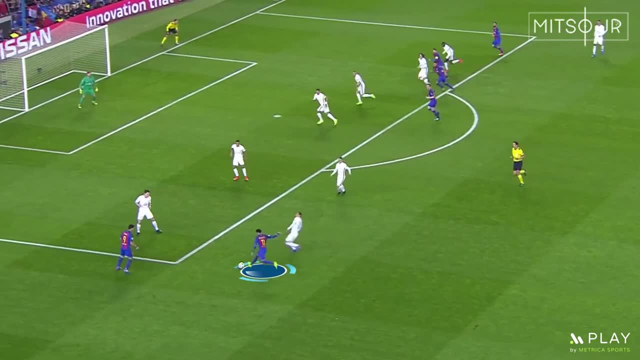 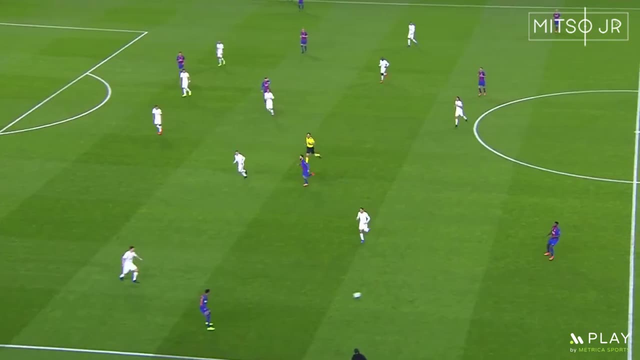 the ball out wide. Just like the first half, he was focused on having the ball under his feet for longer times to try to pull more defenders towards him and then look for passing options inside the block. Now that PSG's defense wasn't that compact, he was able to do that more. 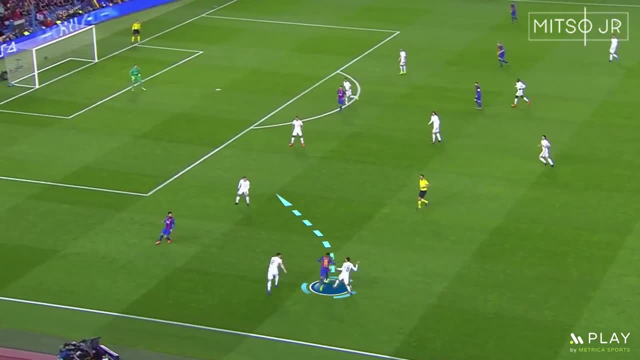 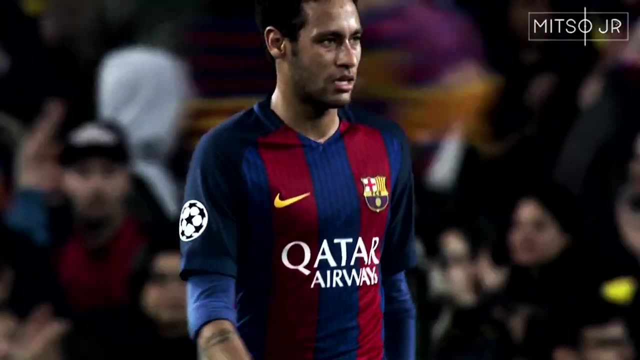 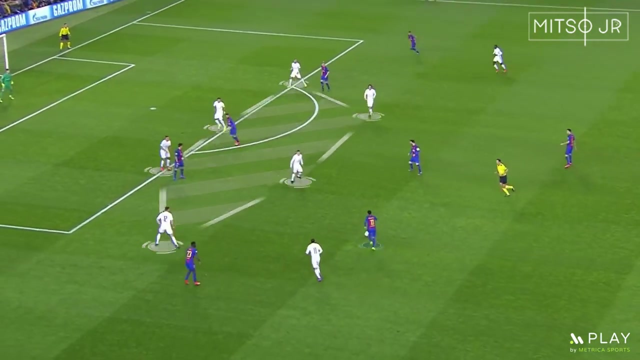 efficiently. Whether he would dribble past an opponent or pass the ball to his teammates, he always moved towards the center and towards the penalty area. Barcelona continued their high pressure. Obviously, every player was giving 110%. Neymar tried to go for long shots again in the second half, but this time no good. 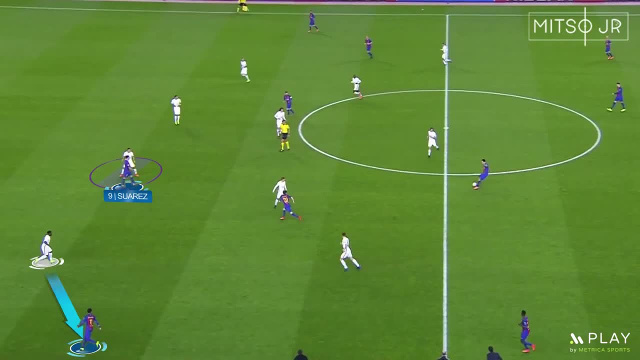 His tactical awareness was seen in those plays where he took the advantage by pulling the full backhand. Neymar tried to go for long shots again in the second half, but this time no good. His tactical awareness was seen in those plays where he took the advantage by pulling the full backhand. 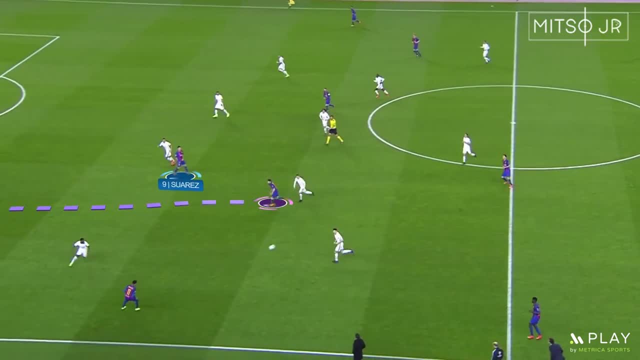 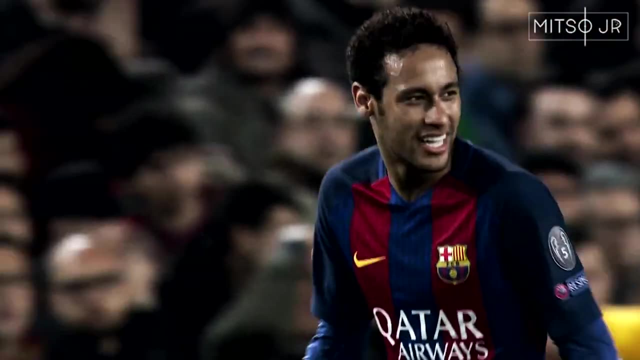 outside, allowing Sergi Roberto here to get the ball in the space between the center back and the full back. He was trying to tactically abuse the four at the back as much as possible whenever the midfielders were not providing the defensive support. Here and after a failed long shot, 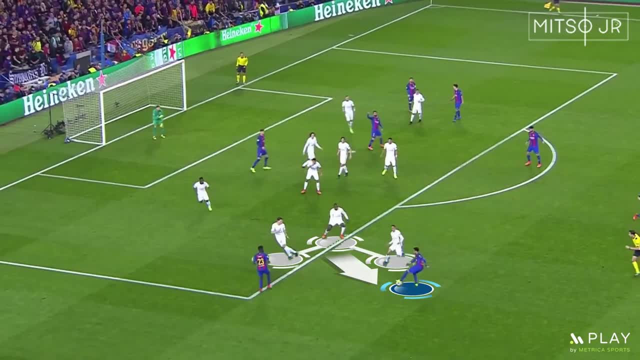 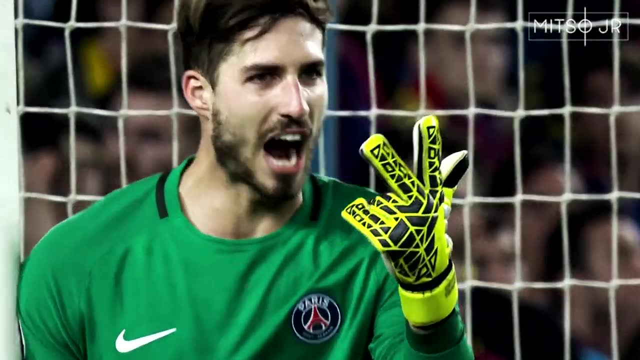 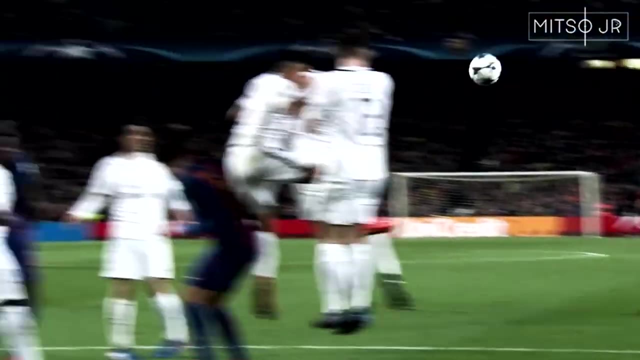 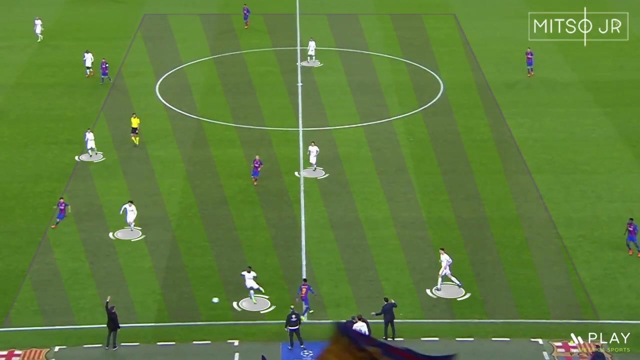 attempt. he sees how the opposition is rushing towards him to block a second shot, so he cleverly wins a foul by covering the ball. You can just see how concentrated he was during those minutes. With no time left, he was trying to outnumber the opposition on the left flank, creating the connection with 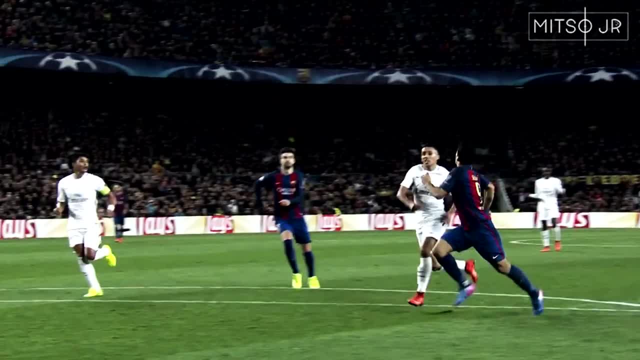 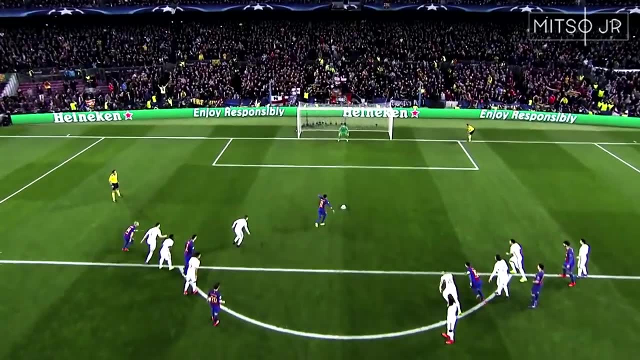 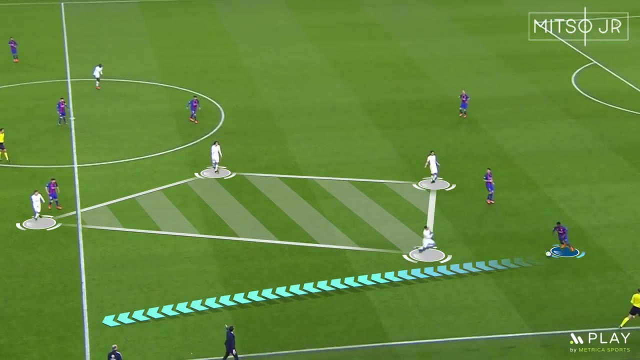 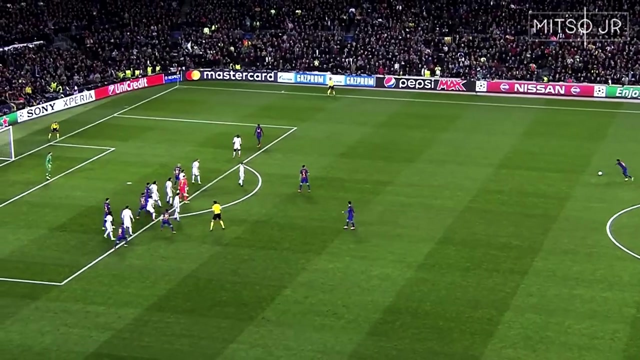 the back line to move the ball on the ground. Luis Suarez was able to win a penalty here and, being the most concentrated player in those minutes, he took the responsibility. He continued to provide options to the back line as PSG applied pressure in the final seconds of the game And finally the magic happened. 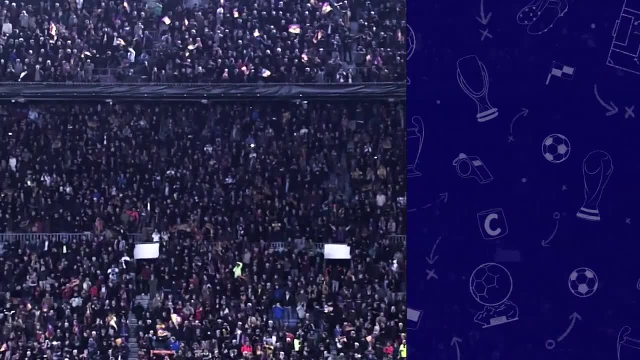 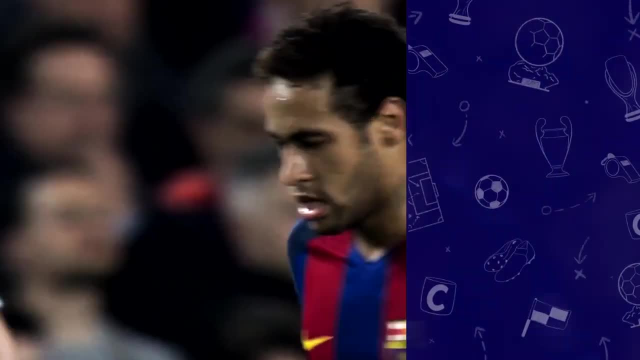 So that was it, guys. I hope you have enjoyed the analysis. Let me know what player you would like to see next. I'll also be uploading a full match analysis for this remontada very soon, so make sure to subscribe so you don't miss out on that video, If you want. 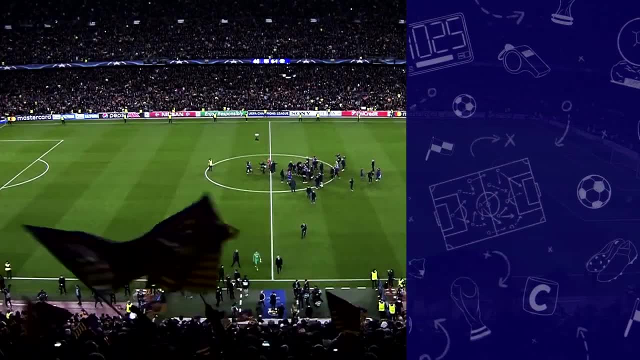 to see an analysis for any other historical match, let me know as well. So thanks for watching and I'll see you guys in the next one. 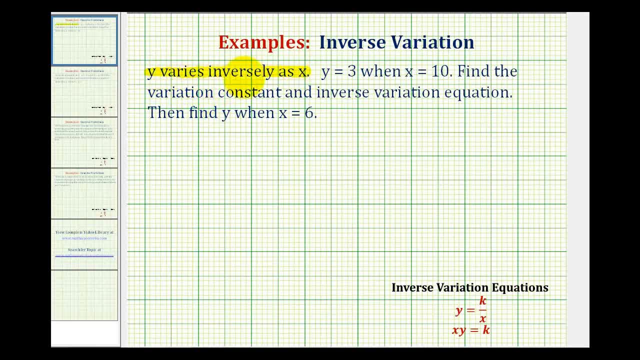 We're given that y varies inversely as x. This is important because it tells us which variation equation to use For inverse variation. we'll be using the equation y equals k divided by x, where k is the variation constant. We'll talk about the second equation in just a moment. 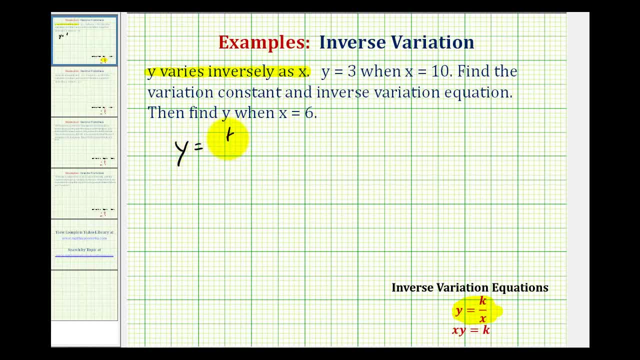 So this problem we'll be using: y equals k divided by x, And then we're asked to determine the variation constant, which is k, the inverse variation equation, and then find y when x equals six. We can find the variation constant because we're told: 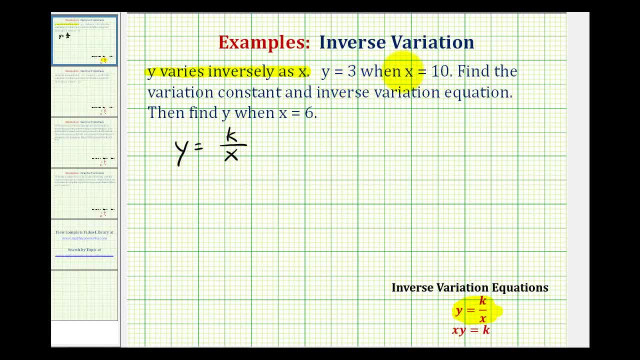 that y equals three when x equals 10.. So we'll perform substitution using these values. So y is equal to three when x is equal to 10.. And now to solve this equation for k, since we have k divided by 10,. 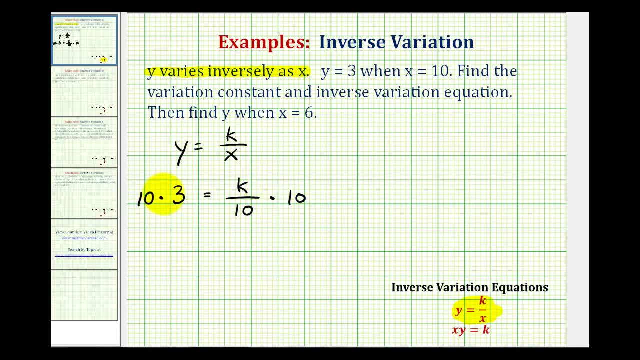 we'll multiply both sides of the equation by 10.. This simplifies to one. so 10 times three is equal to 30, which equals k. or we can say k equals 30. So this is our variation constant. If we take a look at this for a moment, 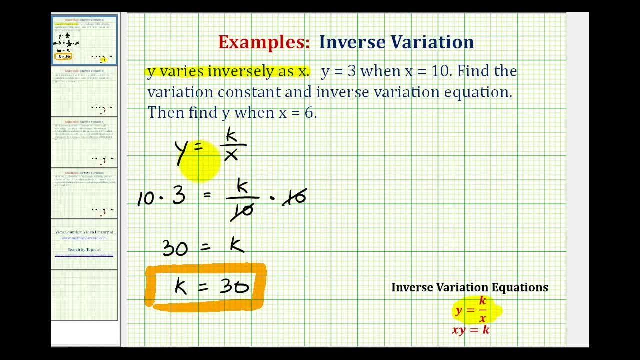 notice how to find k. we multiplied both sides of the equation by x, which would give us the equation: x times y equals k. So we could have found k using this second equation here. So for the inverse variation equation, we're now going to rewrite this equation here.